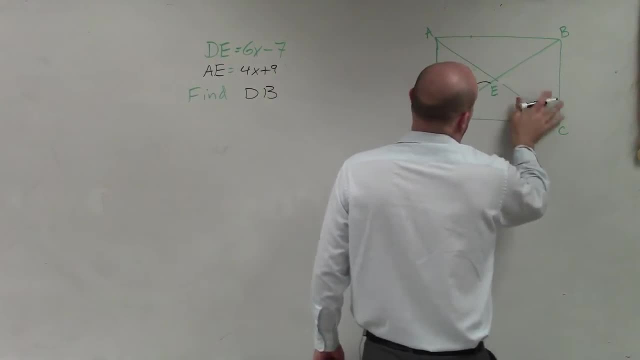 just saying, really it's the same thinking, I'm doing nothing. I'm doing nothing, I'm just saying number four. So AE is 4X plus 9.. Okay, It's really actually going to be the same operation, All right, So then they give us the diagonals, So now we need to go. 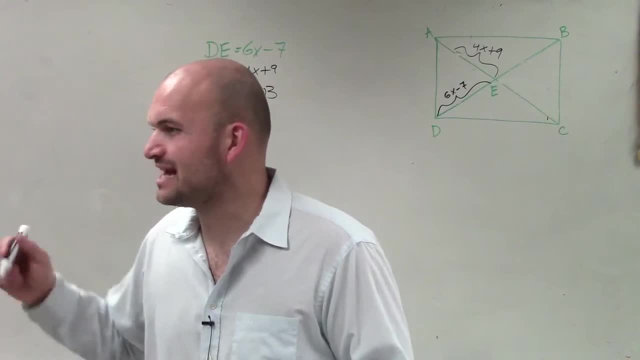 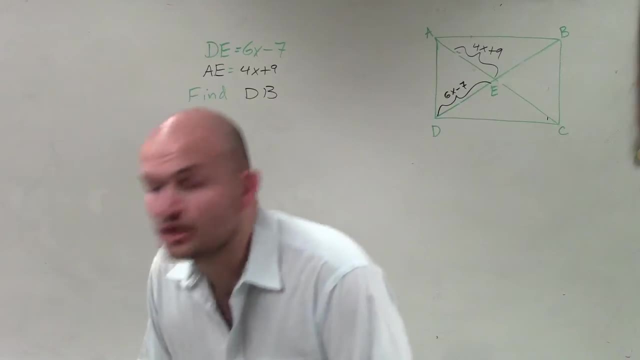 back to our notes and think about: what is it that we know about the diagonals? Do you have your homework out? Write down the problem, because then this is one less problem you guys have to do. Yes, The diagonals are congruent, right? Do you guys remember we talked about 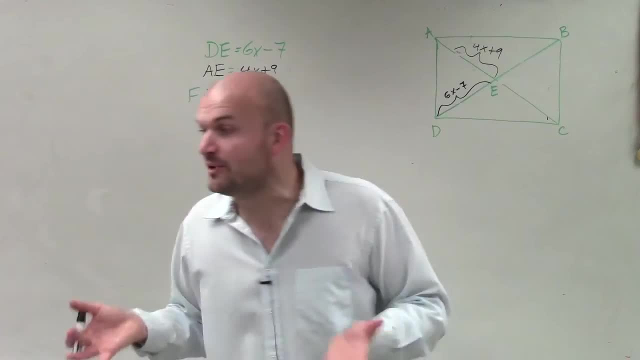 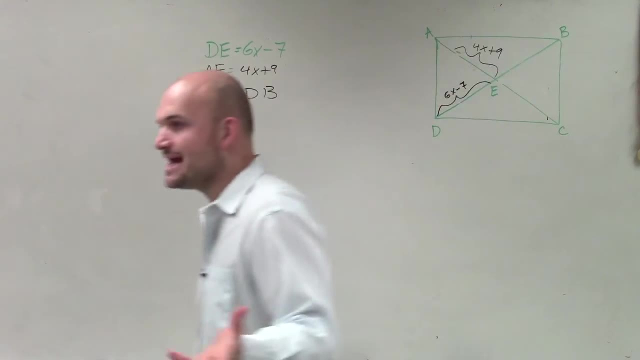 that. That was the one condition. That was the only thing new that we went over last class period. Diagonals for a rectangle are equal in measure. Besides that, a rectangle has all the other properties of a parallelogram. So now we got to go back and think: all right, well what? 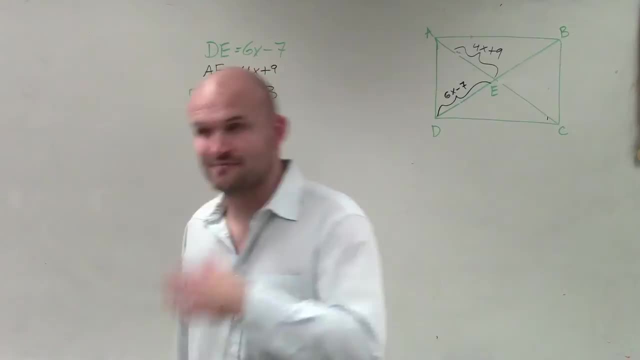 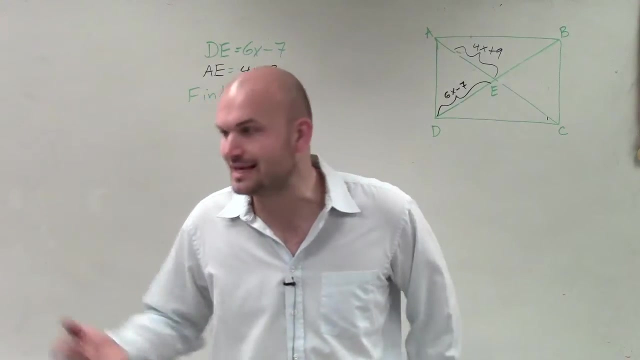 were the properties of a parallelogram for the diagonals. So you have to go back to notes for two days ago and think about all right again. what did the diagonals do right For a parallelogram? how are the diagonals related to each other? Now, so one. we know that this. 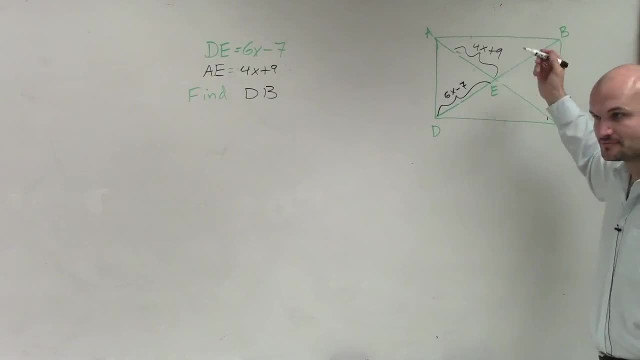 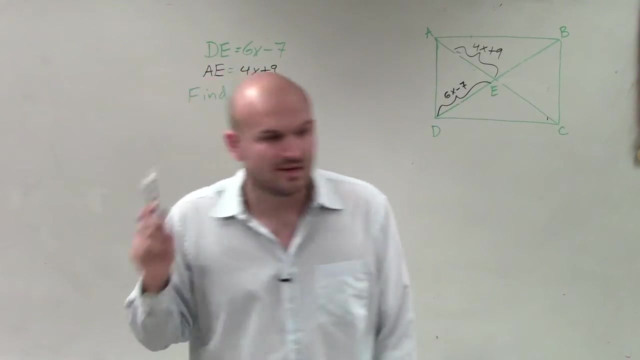 diagonal is equal to that diagonal right. There is also one met, one else one, something else that's very, very important about the diagonals of any parallelogram. Seth, I'm going to have to have you either put that face down on your desk, put a pen or pencil in your 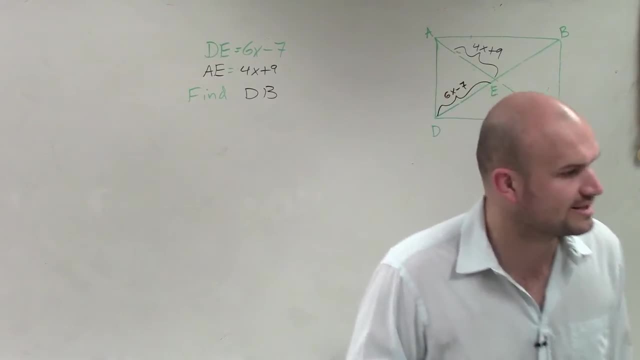 thing, or we're going to have some problems. because you need to be paying attention to watch this. write this down. Does anybody remember what else was about parallel? what else about the diagonals? We know, in a rectangle the diagonals are equal to each other, but 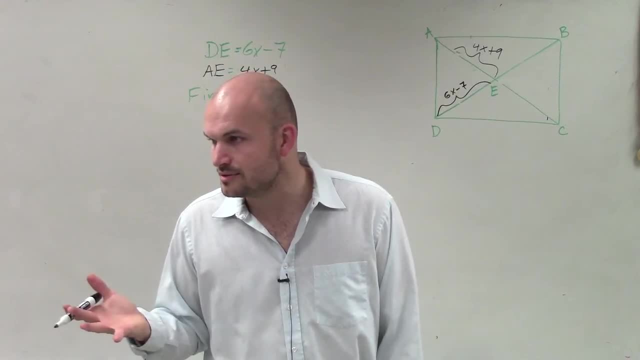 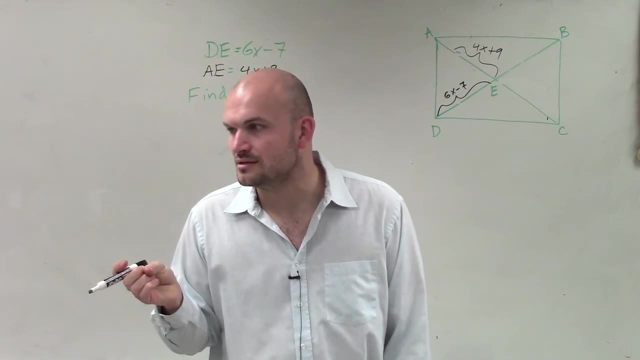 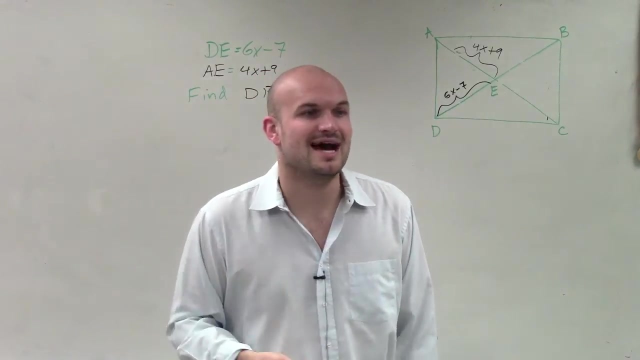 there's one more extra property, Zach, do you remember? Huh, Think about the diagonals. just the diagonals, Elizabeth. No, What about the diagonals? Something that rhymes with tisection. yes, They bisect each other right, They cut each other in half. So let me ask you this question. 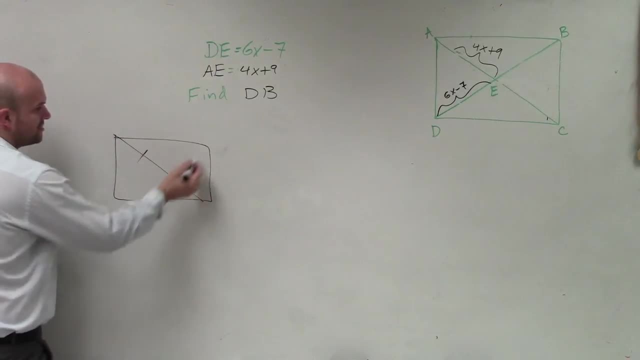 If this right, that whole side is equal to that, this is equal to that, and if they cut each other in half, okay, well, let me do that. So this diagonal is equal to that diagonal right, That's per a rectangle. We also know: 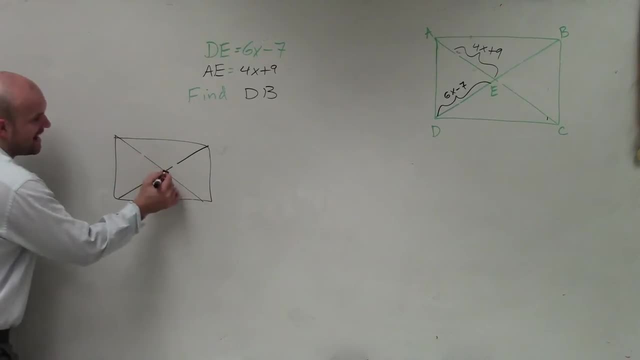 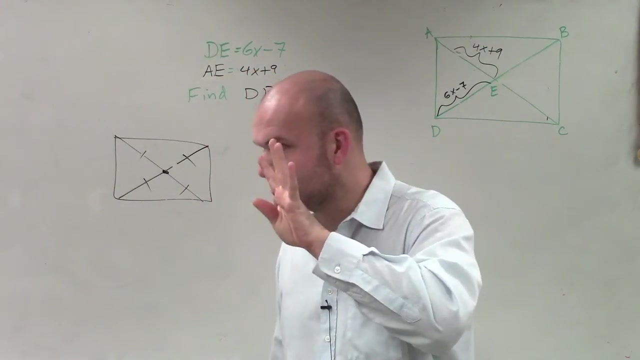 per the parallelogram that this side bisects this side and this diagonal bisects this one. Well, if they're both equal in length, then when you cut them all in half, you have four equal lengths. Does that make sense? Does that make sense? Does that make sense? 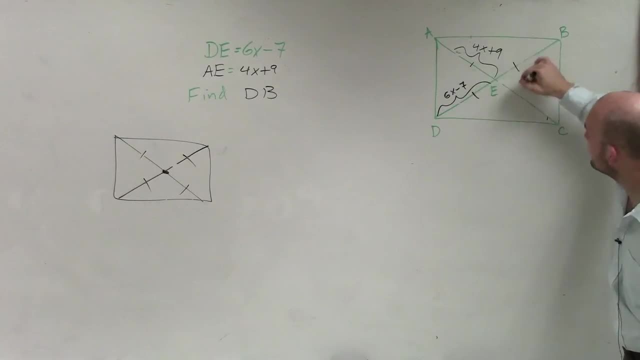 So guess what, guys? These all are equal in measure for all rectangles. So if they're equal in measure, equal, equal, that means we can set an equation. So now I can say: 6x minus 7 is equal to 4x plus 9.. Now I have an equation. Now I can find the value of x. 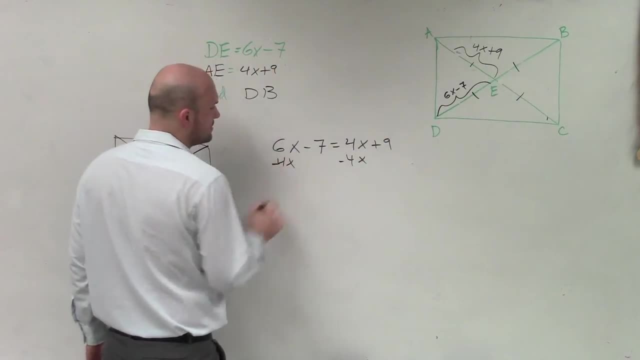 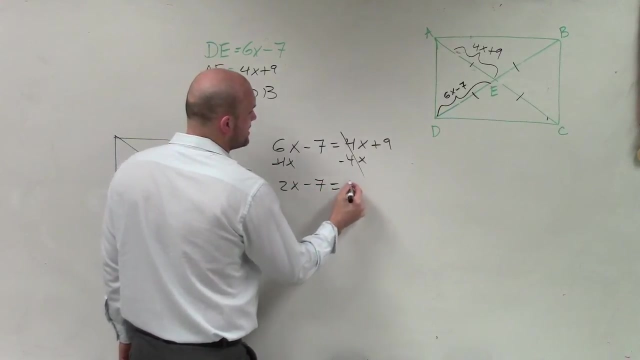 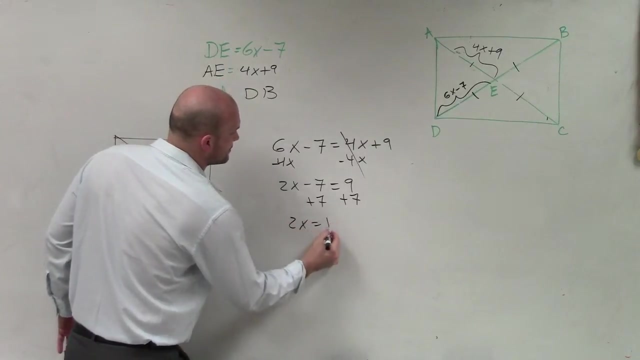 So I subtract 4x on both sides using subtraction property of equality: 6x minus 4x is 2x minus 7 equals 9.. Now I can use my two-step equation, use my inverse operations and I have 2x equals. 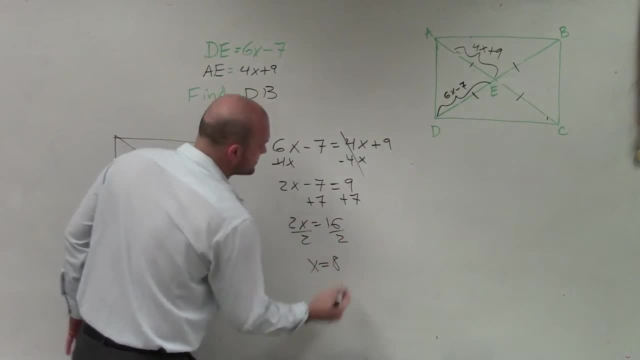 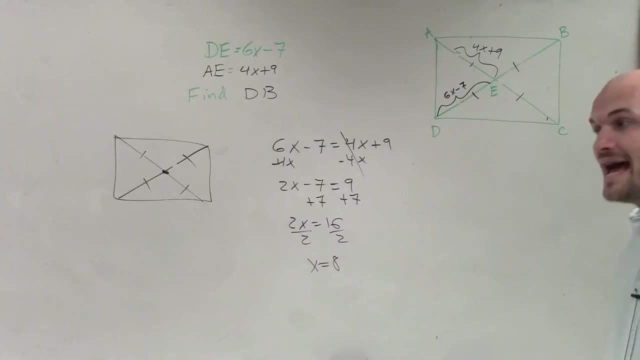 16,. divide by 2, divide by 2, x equals 8.. All right, but that's not what they asked, right? They said what is the length of db, not what is x. Well, if this guy's a 6x minus, 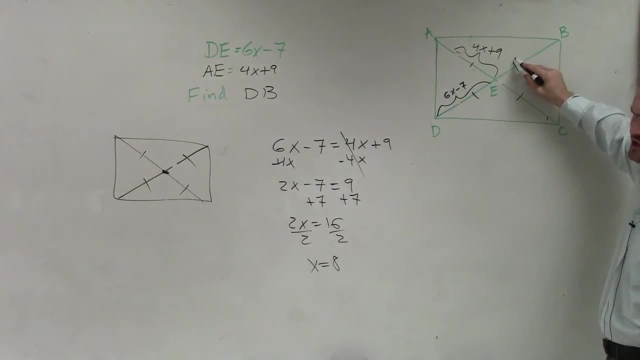 7, and this is equal to this. what does this length have to be, as far as an expression, 6x minus 7.. Right, So really the length of db is equal to 2 times 6x minus 7.. Would you guys agree? 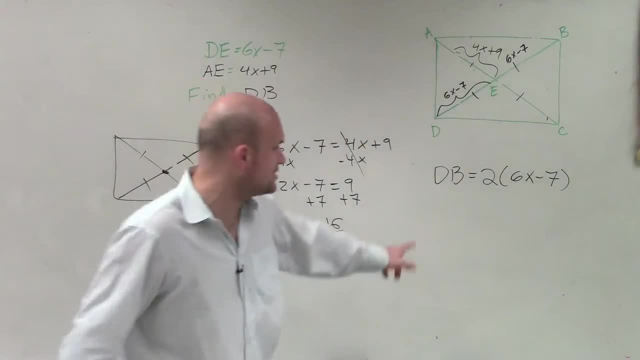 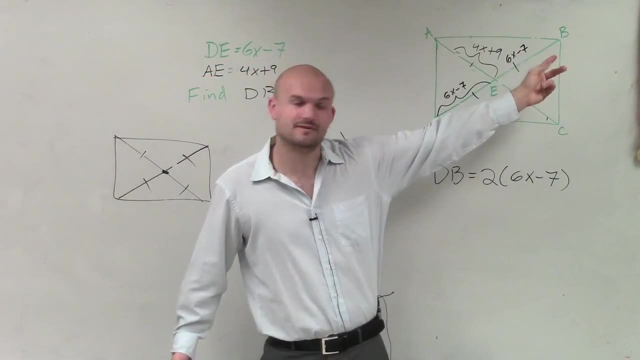 about that. I could say 6x minus 7 plus 6x minus 7,, but you could also write it like this: It's two of them, right: 6x minus 7 plus 6x minus 7, or 2 times 6x minus 7.. Well, 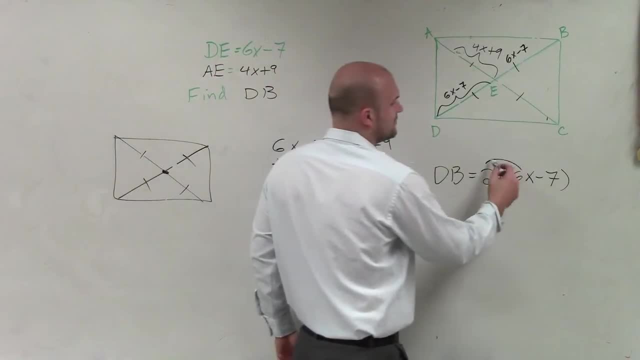 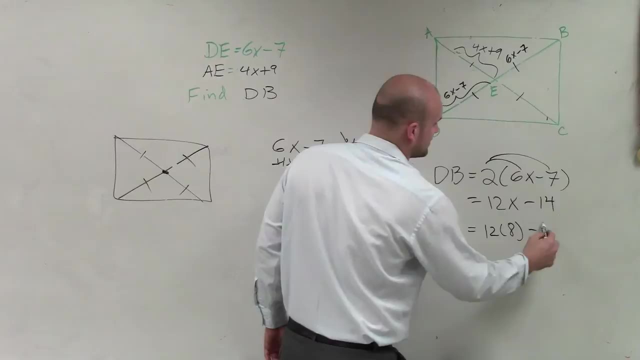 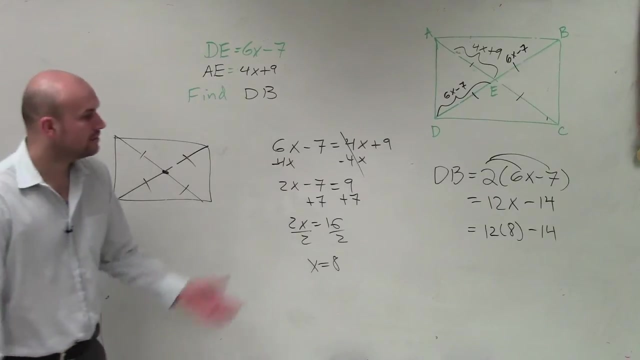 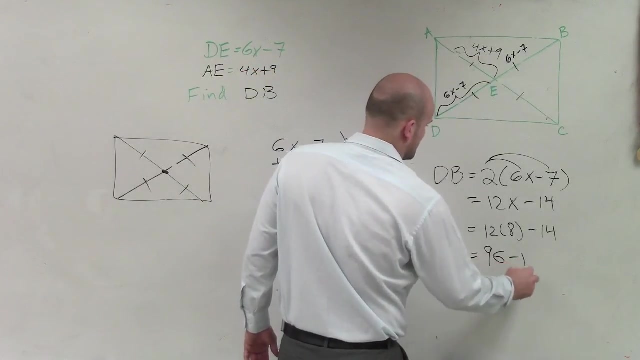 now I know that x equals 8.. So first thing I'll do, though before I do that, I'll go apply distributive property. So I have 12x minus 14. Then I have 12. So 12 times 8 minus 14. Okay, Cool. So 12 times 8 is going to be 96. And then this will: